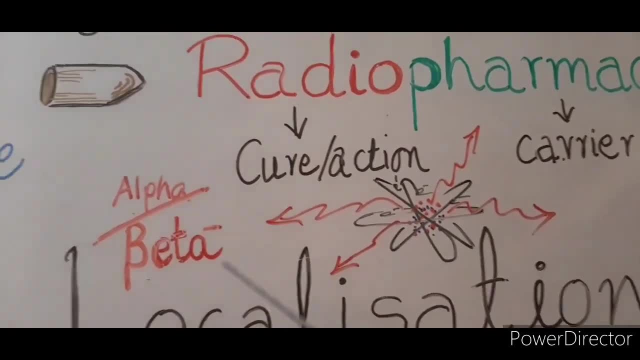 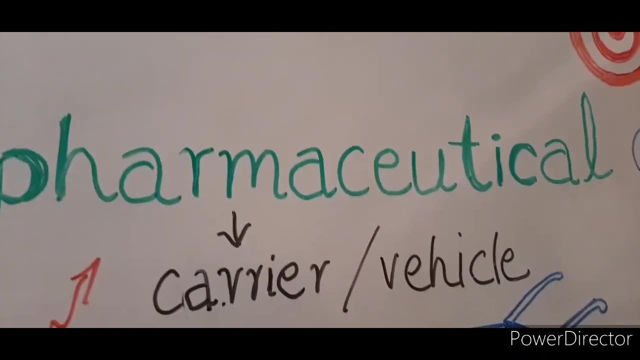 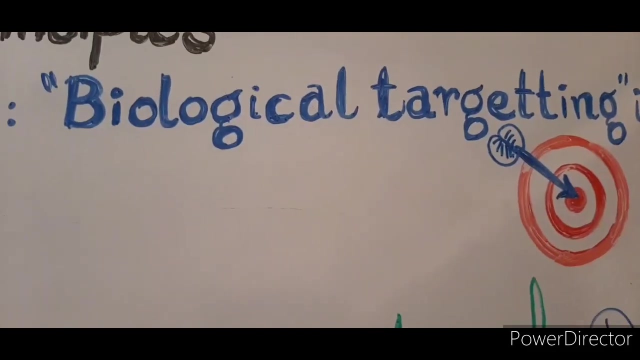 radioactivity Radiations, nuclear radiations. Now these radiations are carried by the carrier or vehicle. that is the pharmaceutical to go specifically to the region of interest, and that is what is biological targeting, That is, only the undesirable cells, mostly the cancer cells. 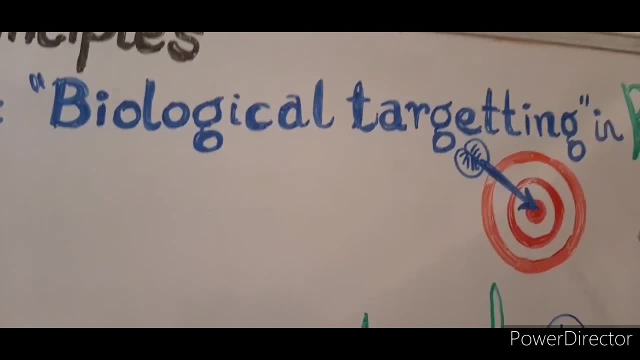 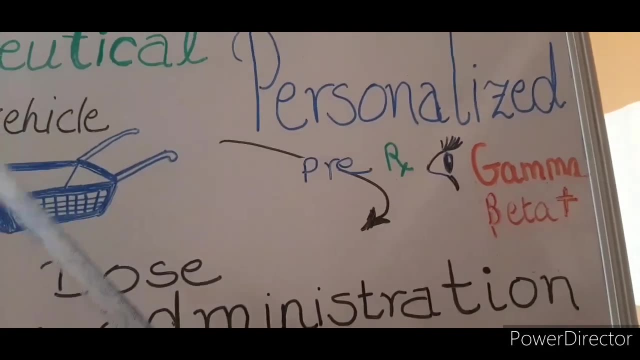 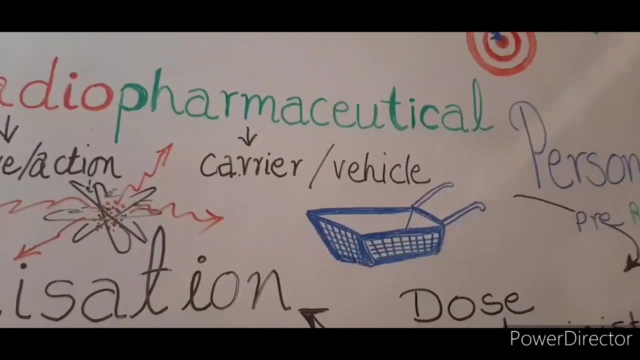 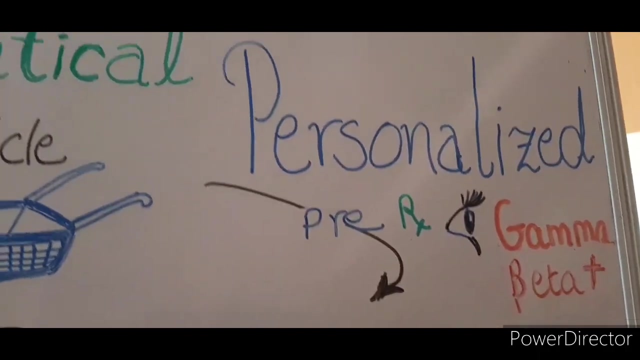 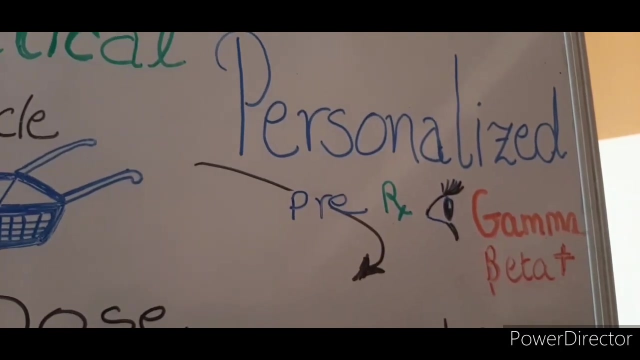 are killed and the normal tissue is spared. This kind of personalized therapy is because of the specific action of the carrier vehicles towards the region of interest against cancer cells. Now the pre-therapy scan can be performed using gamma or beta plus sources, which are signals now just like any diagnostic procedure, and this can act as a map or a treatment planning. 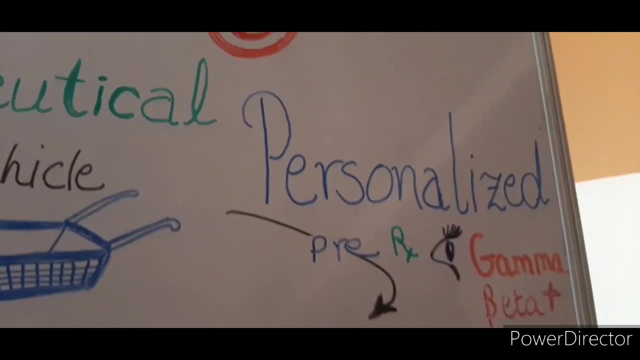 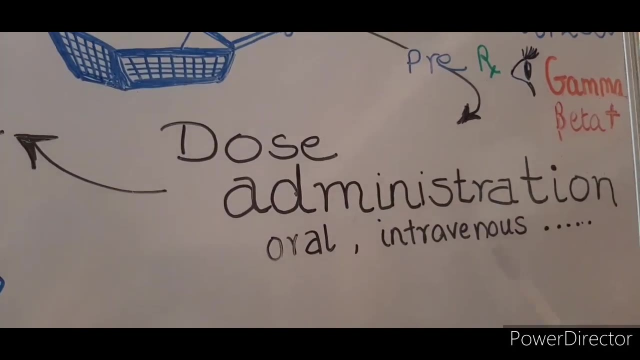 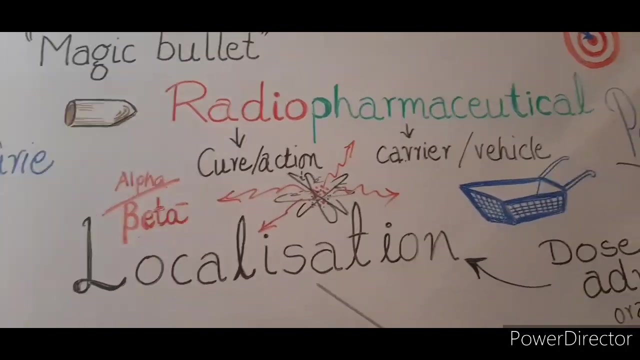 tool. Once the treatment has been planned, dose is administered in the form of oral or intravenous route and any other route, these two being the most common. The therapeutic radiopharmaceutical localizes into the region of interest and does the needful. However, the patient 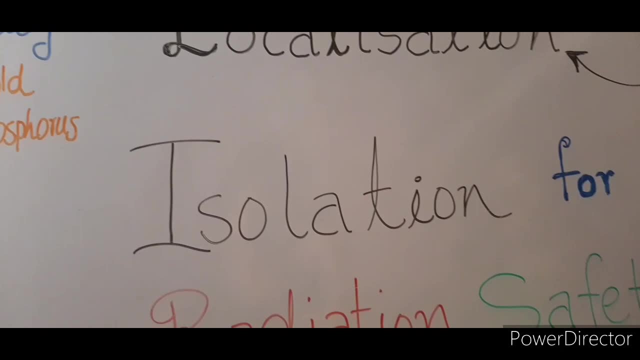 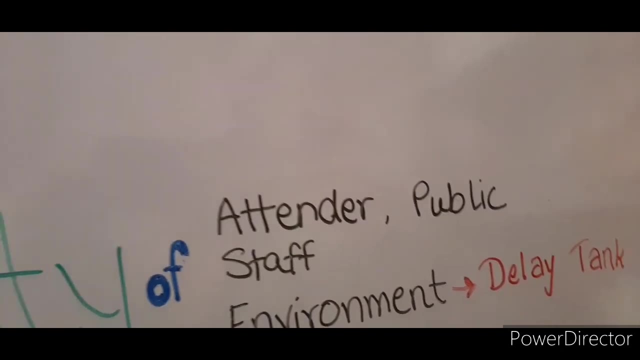 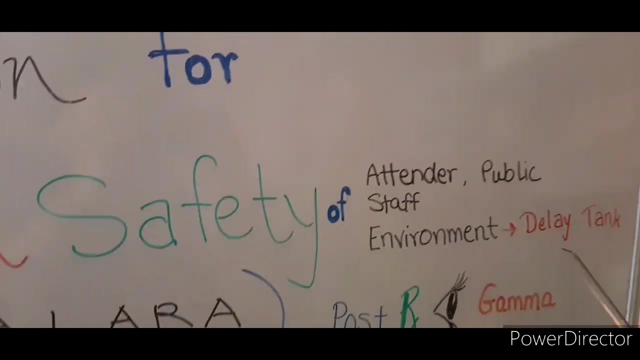 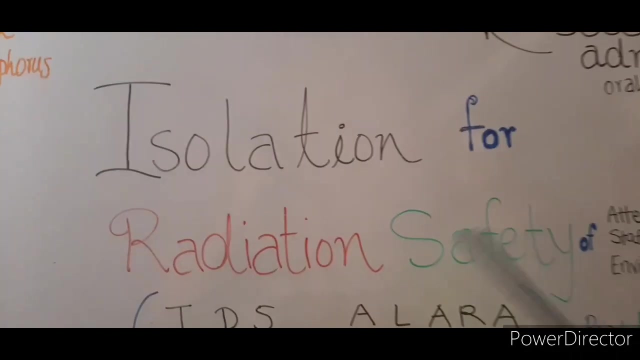 who is radioactive has to be isolated for the radiation safety of the attender public or staff. even the staff And even the effluents which are produced from the patient has to be sent to the delay tank for the environment safety. The golden rules of radiation safety are the minimum time that has to be spent with radioactivity. 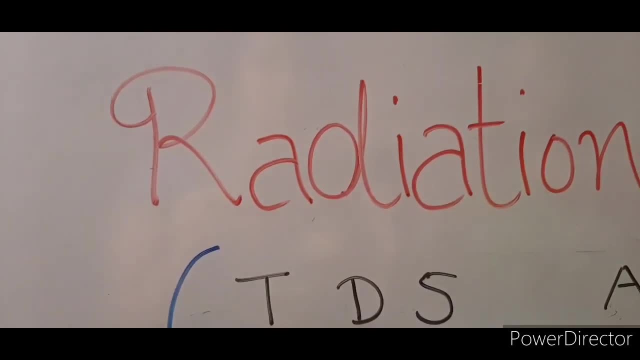 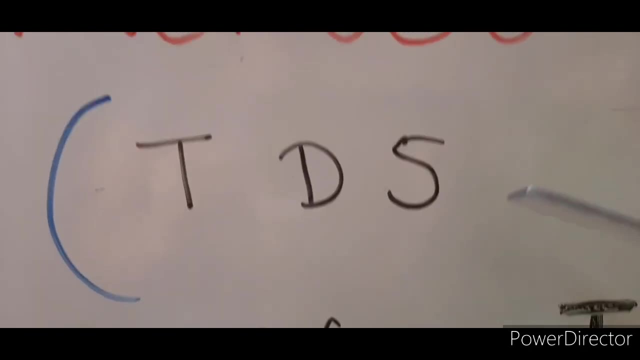 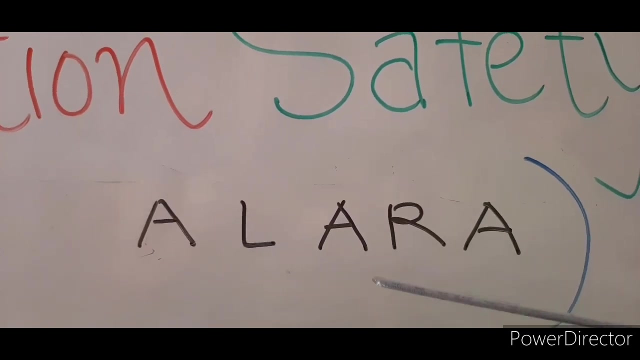 and that is the radiation source in this case the patient's also, the maximum possible distance from the patient. that is why the isolation and the shielding like apron or gloves and so on, And the golden principle, that is, the practically possible, as low as reasonably or practically. 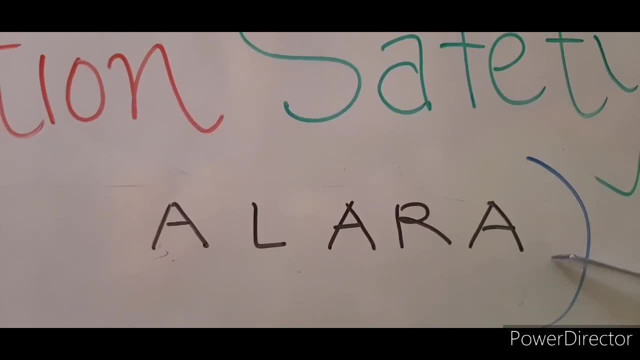 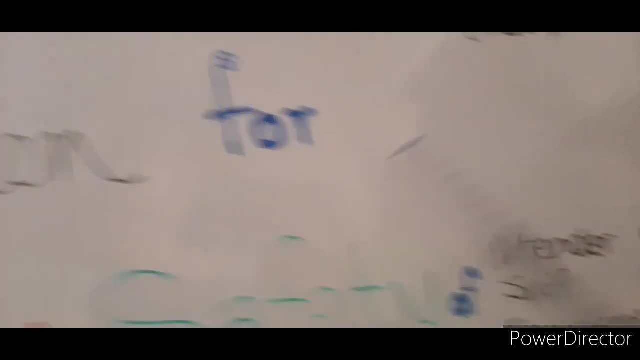 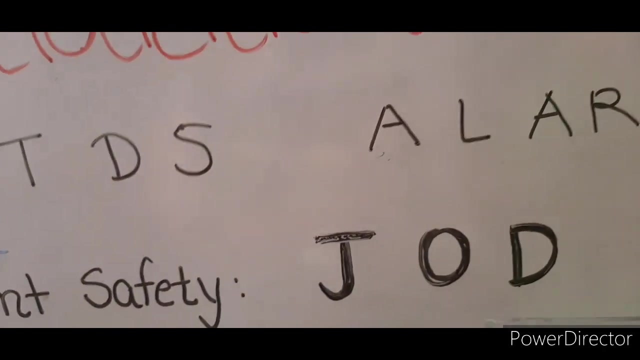 achievable exposure levels. minimizing- that is the, for example this attender has- is a must in case of pediatric cases. isolation. Now here we have to understand that even the patient's safety has to be considered, that is, the referring doctor and nuclear medicine physicians. And to continue the same principle, in this case we use this famous principle of JOD that